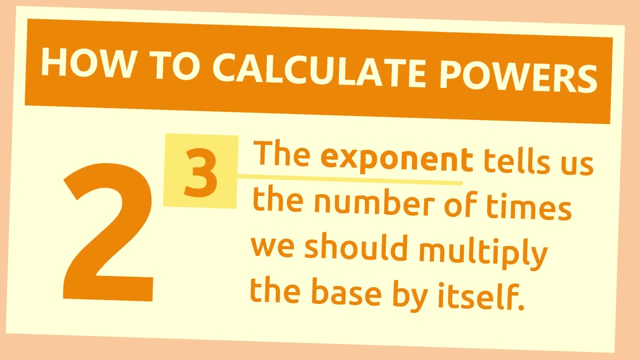 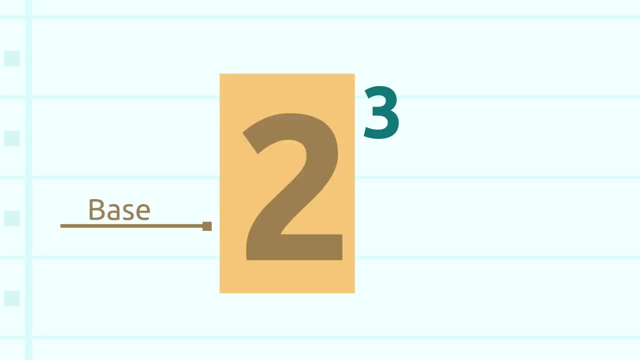 multiply the base by itself. Let's look at the example we have on the screen: Two to the power of three. As we said before, the base of this power is two and the exponent is three, which is the number of times we should. 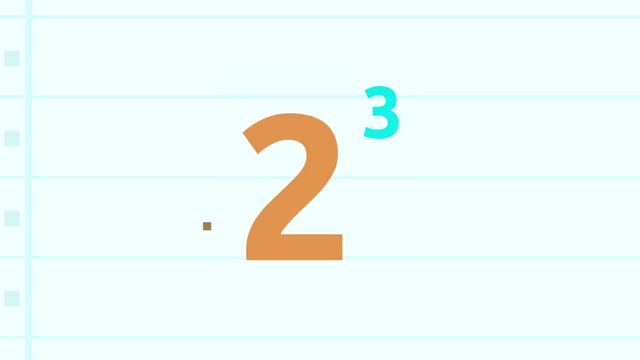 multiply the base. So two to the power of three is two times two times two, which equals eight, Meaning that two to the power of three is eight. The result of this multiplication is called power Easy right, Let's look at another example. This one is easy: Three to the power of four. What do we need to do? 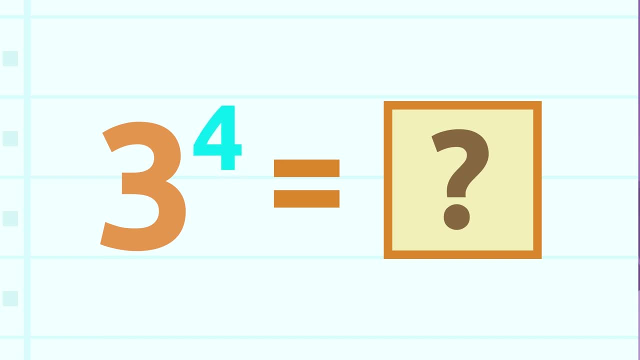 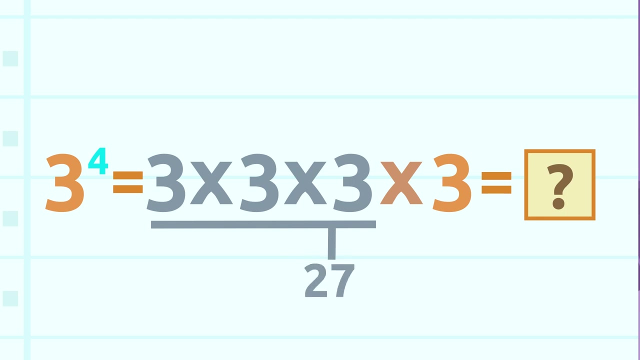 We need to multiply the base by itself, the number of times indicated by the exponent. This means that we should multiply three by itself four times. Let's look at the result: Three times three times three times three equals. Hmm, it's better to multiply separately. 3 times 3 is 9.. 9 times 3 is 27.. And 27 times 3 is 81.. Awesome. 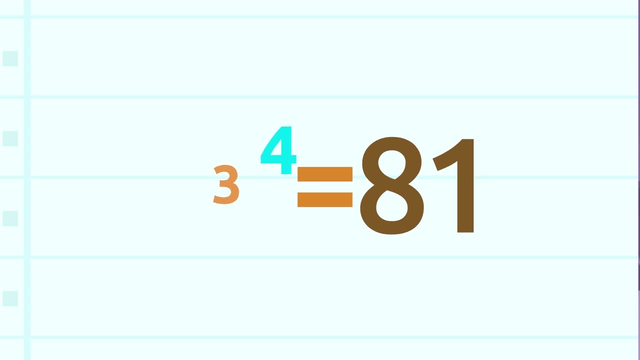 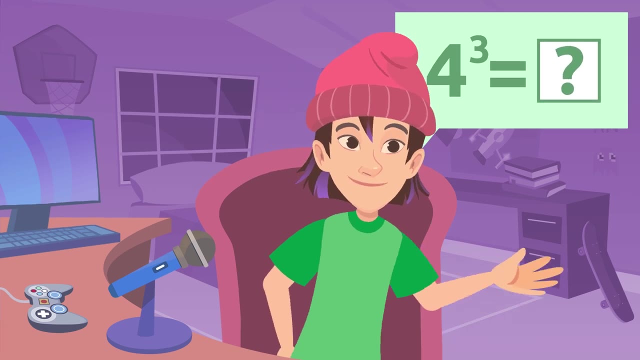 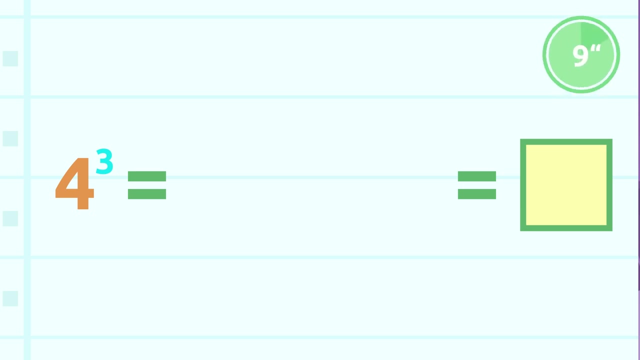 3 to the power of 4 is 81.. Would you like to try doing one yourself? Calculate this power: 4 to the power of 3.. Time's up. Do you have the answer? Let's see. to calculate 4 to the power of 3,. 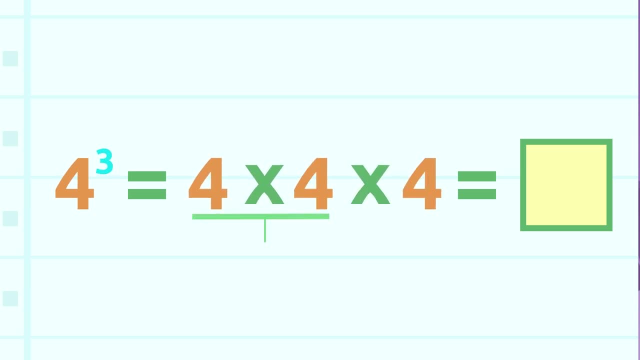 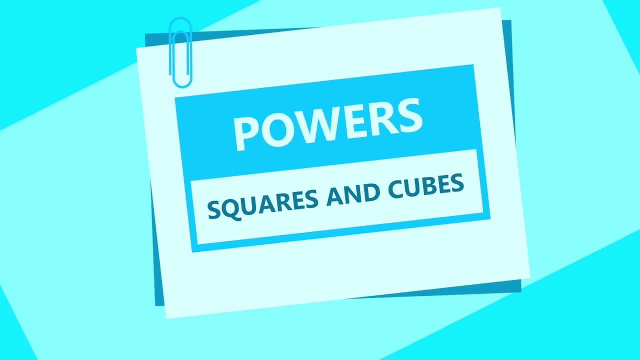 we should multiply 4 by itself three times. 4 times 4 is 16, and 16 times 4 is 67.. is 64.. 4 to the power of 3 is 64.. Well done everyone. Here's a little secret, Did you know? 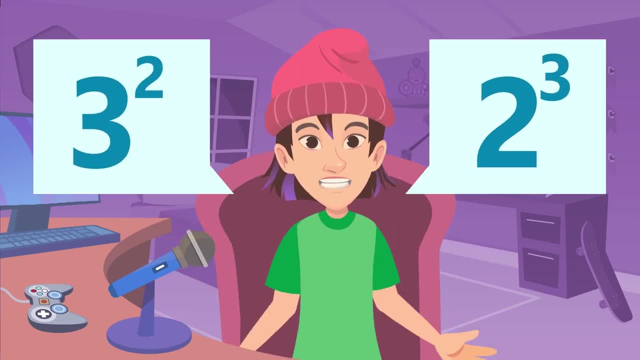 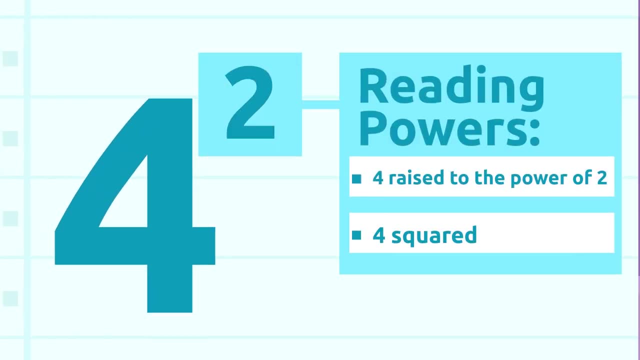 that when a number is raised to the power of 2 or 3, it can be read differently. When a number is raised to the power of 2, we can also say squared Here, for example, 4 raised to the power.